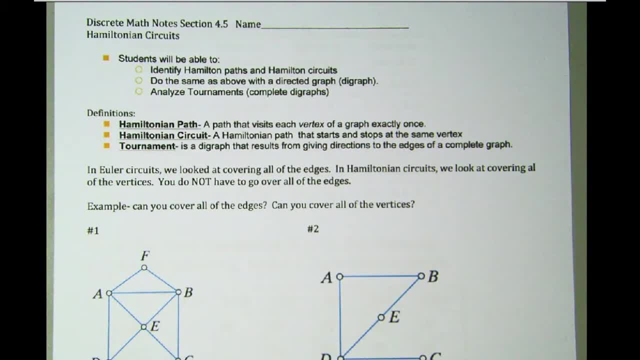 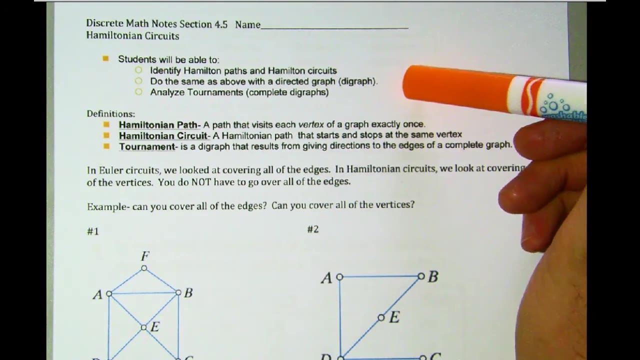 All right, this is discrete math notes, section 4.5. Hamiltonian circuits. Previously we did Euler circuits, Now we got to figure out what this Hamiltonian circuit thing is, And so what we want to be able to do is identify Hamiltonian paths and Hamiltonian circuits and do the same for a directed graph. 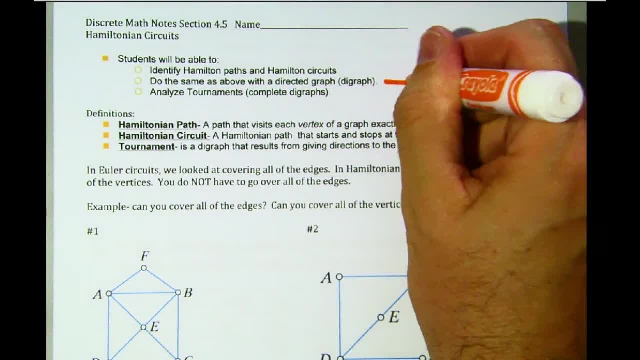 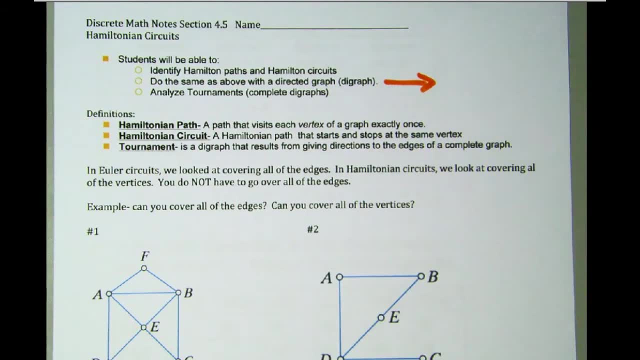 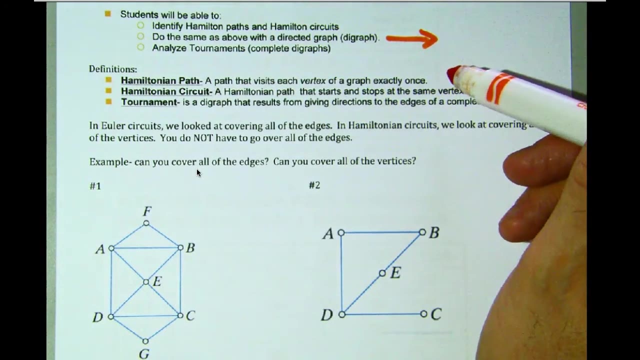 which is a diagraph. When we have a directed graph, we have arrows, not just segments. And then we want to analyze tournaments, which are complete diagraphs. So some definitions: Hamiltonian path, Path that visits each one of the vertices of a graph exactly once. That's. 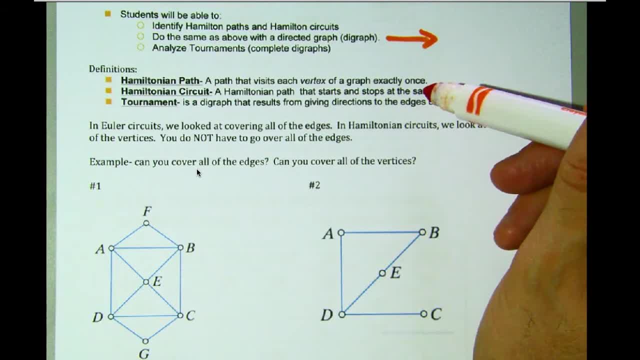 what we want to do. Go to each vertex, each, exactly one. The circuit visits each vertex and starts and ends at the same vertex, And then a tournament is a diagraph that results from given directions to the edges of a complete graph. so previous section: we did Euler. 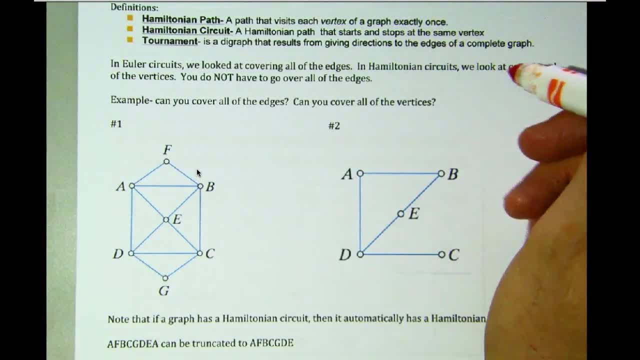 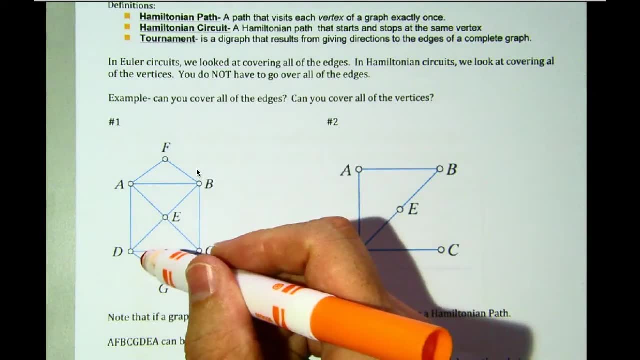 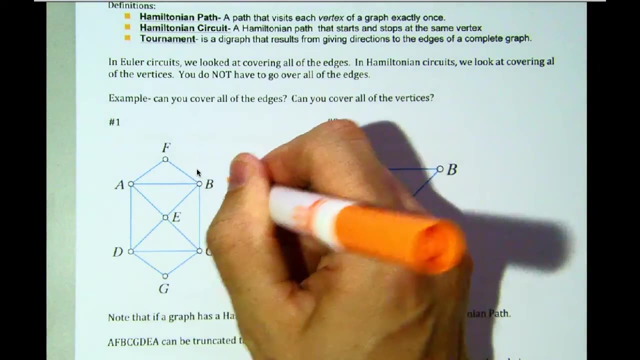 circuits. we wanted to cover all the edges and finish back to where we started from, so let's try that. if I did an Euler circuit here, is that possible? remember we count the number of degrees: one, two, three, four. one two, three, four. one two, four, four. so all of these are four, these are two, and so all of them. 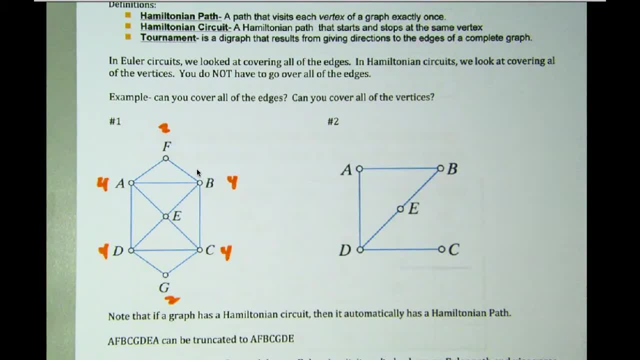 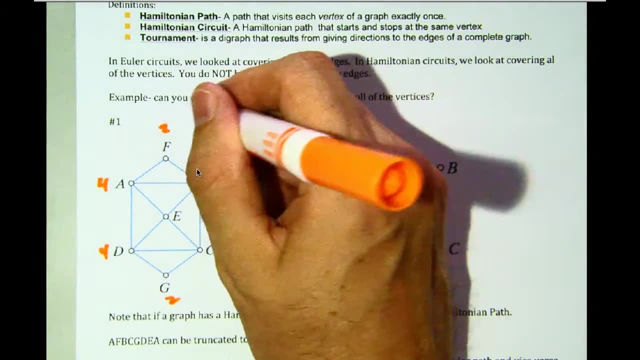 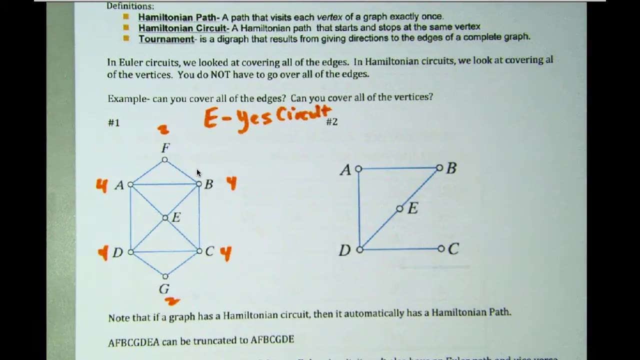 are, even if all the vertices are even degree, in other words, they have this, the even number of edges that come into it. then, yes, we can make an Euler circuit if it's an Euler path, that is only if we have exactly two odd degree vertices. so you got to remember that. so Euler, yes, and so if I do this, I'd have to zip. 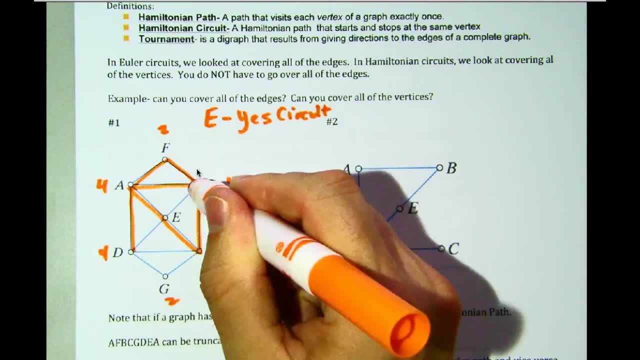 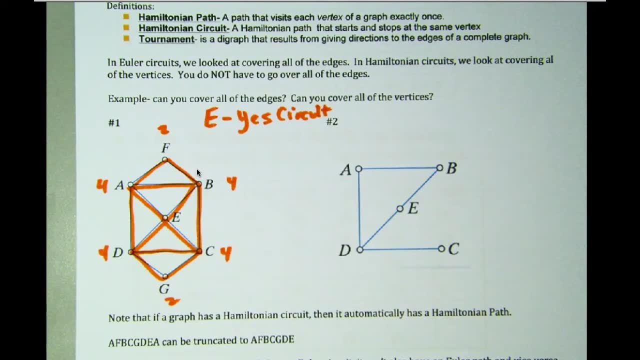 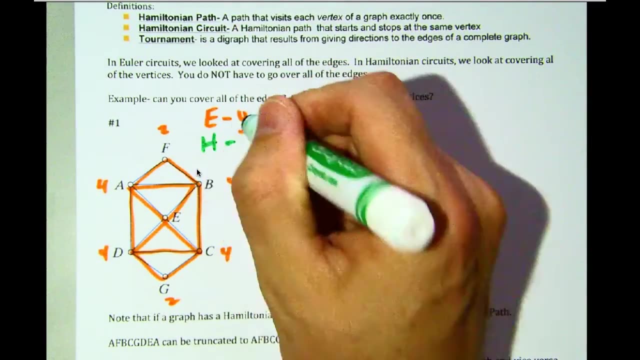 around you, you, you. there's my Euler circuit. now I don't know if you want to do that or not, because we did that previously. now I'm gonna draw on this because I want to do a Hamilton, Hamiltonian path, Hamiltonian circuit. now, what happens with this is: 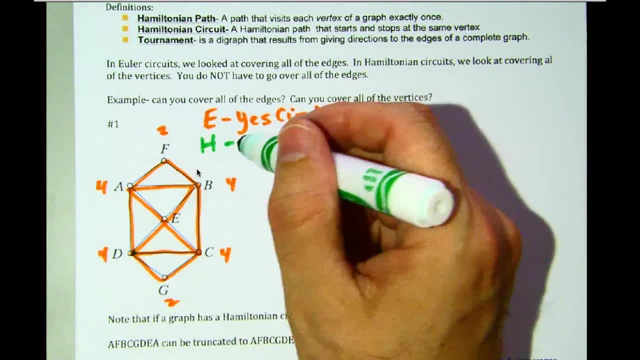 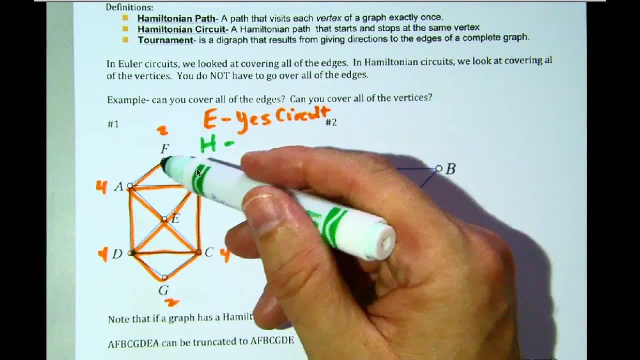 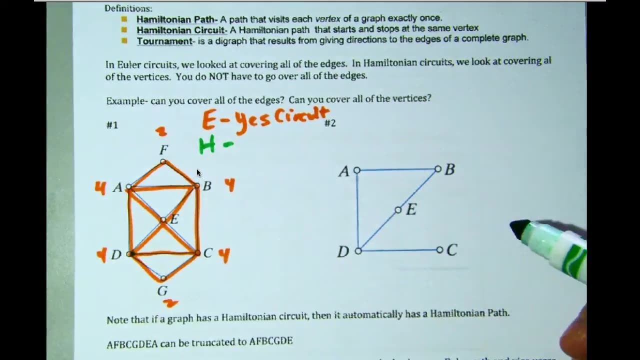 that if I start here, I just want to, by the way, I just want to cover each vertex. so the difference is here: is Euler circuit? is a Hamiltonian circuit? Euler might be like the snowplow going through each one of the streets and plowing each one of the streets the Hamiltonian is representative of, possibly. 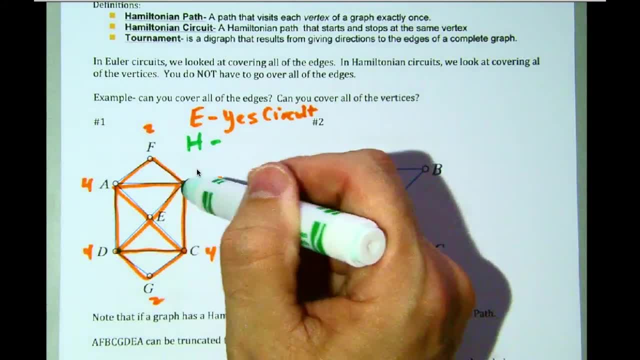 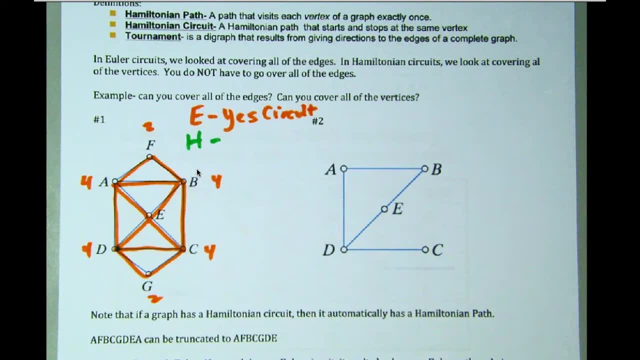 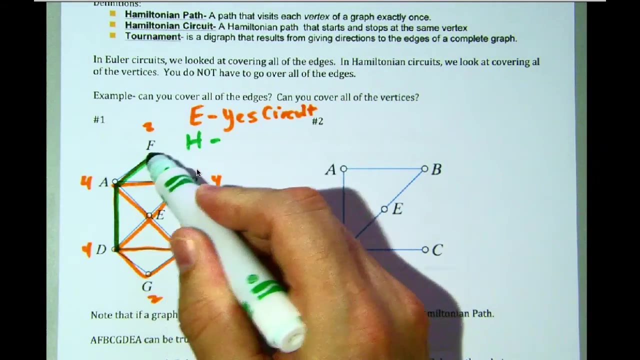 a delivery person. you want to go and deliver to each one of these places and you probably want to minimize actually how many streets that you cover. so you don't want to cover all the streets if you don't have to. so if I start here, I can go to a. 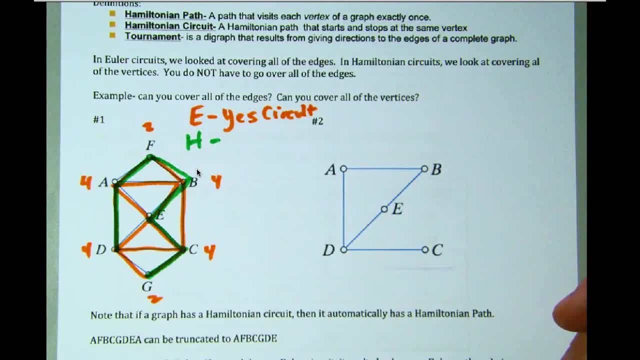 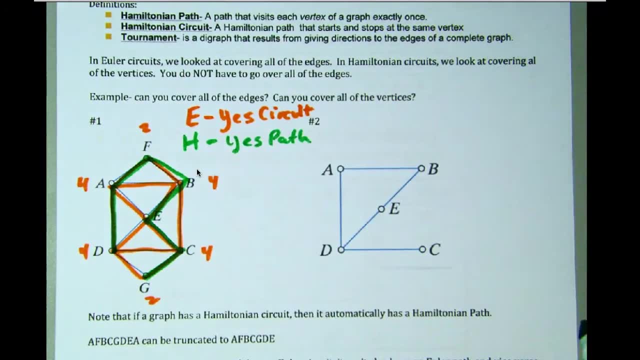 now, if I stop right there, that would be a Hamiltonian path. now, what's different about Hamiltonian is that Hamiltonian can be, yes, just path, and yes to circuit. with Euler it was one or the other. with Hamiltonian it can be both, in fact, if you. 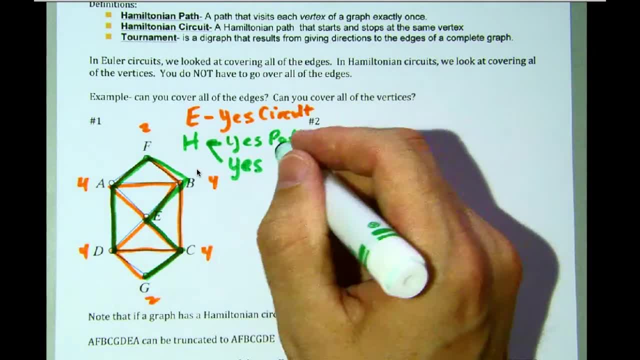 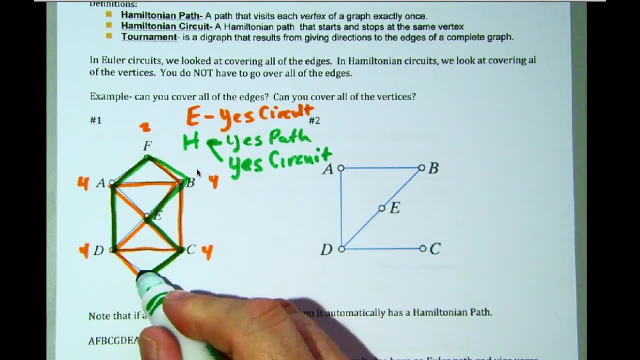 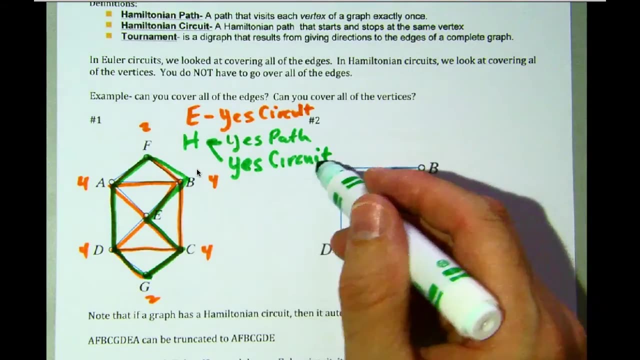 have a circuit with the Hamiltonian, you also have a path, because you just stop one short. so here I stopped at gee. can I finish this up and go back to G, where I started from? yes, I made all my deliveries and I can go back home. that's what the circuit does and for the 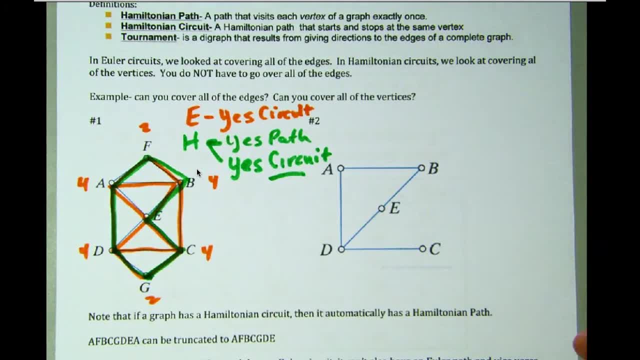 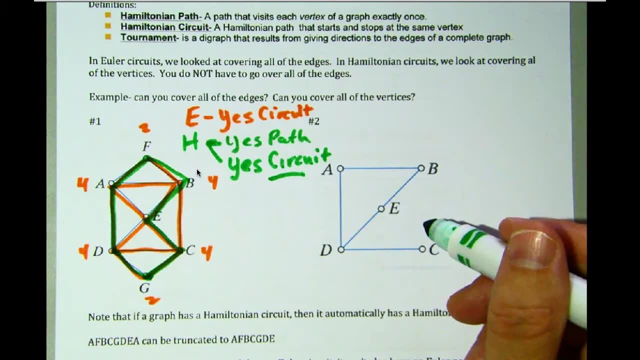 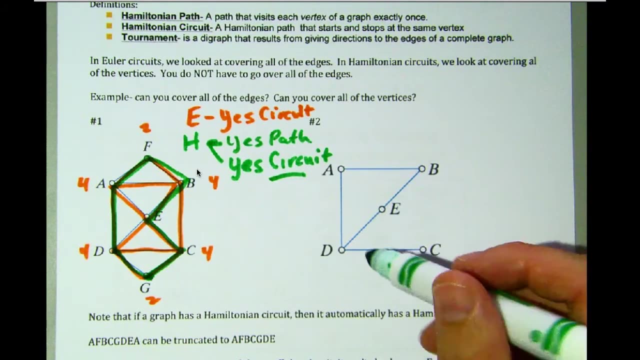 path. it was just stopping one short. okay, now if I look at this one, can I do an Euler path with this, or an Euler circuit? well, if I start here, I'm not gonna be able to finish here. this is odd, and this one is odd degree, and so what has to happen is that, for an oiler, I'd start at. 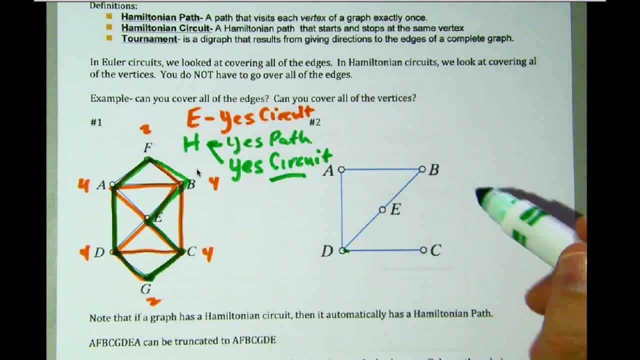 C and finish at D. now what about if I wanted to cover all the vertices? I'm going back to Hamiltonian again circuit, yes or no? well, I don't think so. I can't really start and stop at the same spot without duplicating one of these edges. 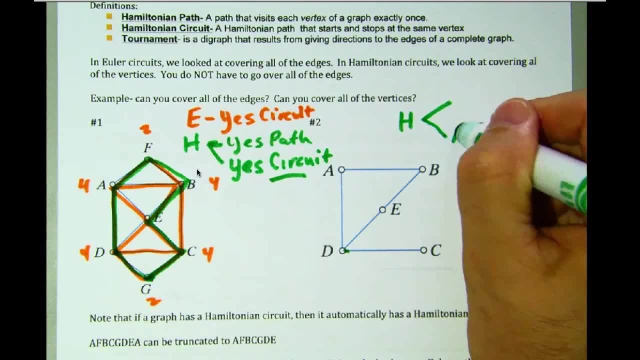 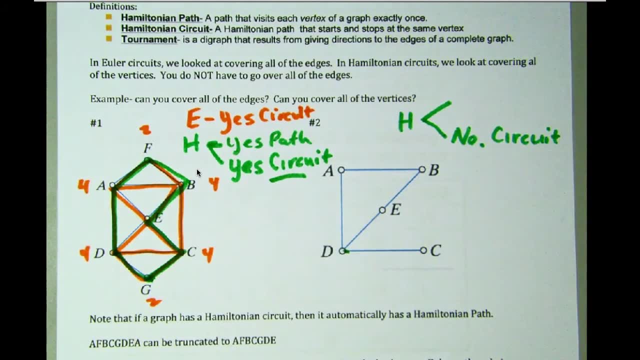 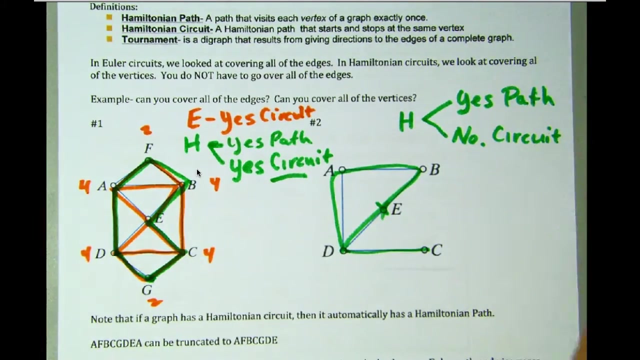 so with this, the Hamiltonian circuit is a no, no to the circuit. but what about a Hamiltonian path? sure, I can do this and I can do that. that would be. I'm sorry, I just need to stop there. so this would be yes to a path to make this a circuit. I would somehow somehow have to go back. 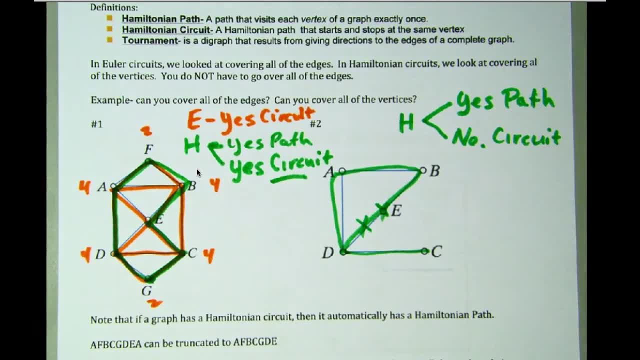 home. so this you right here. I didn't need for that to be a path. I could have stopped right at E all. right now with the Hamiltonian circuit you're gonna have a lot fewer edges covered than you did with the oiler, just by the nature of the. 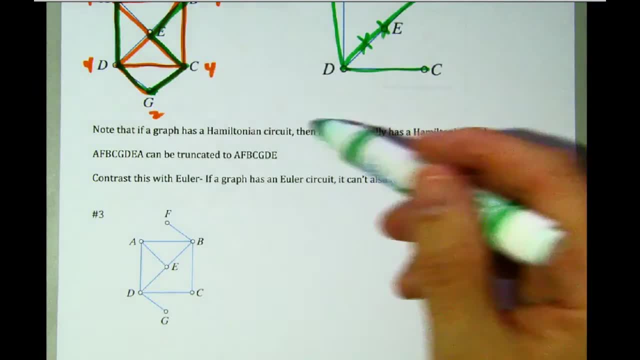 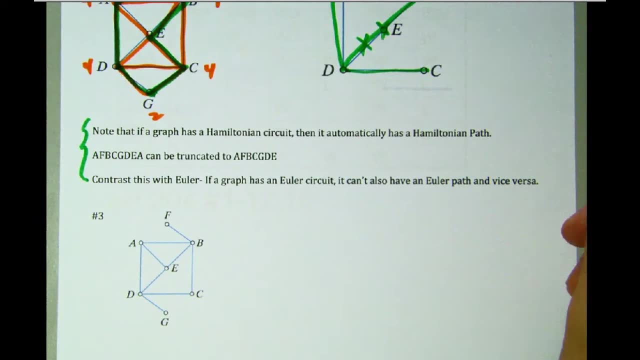 definition. so if you look at what I have written right here, please read that. but it really it reiterates what I just said about a Hamiltonian path. if I have a Hamiltonian circuit, that I have a Hamiltonian path if I have Euler, Euler is one or the other, you can't have a circuit that. 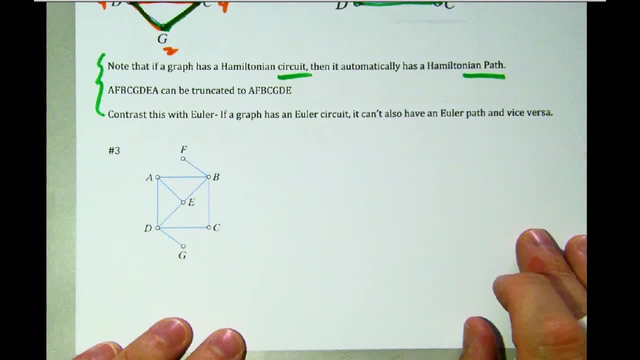 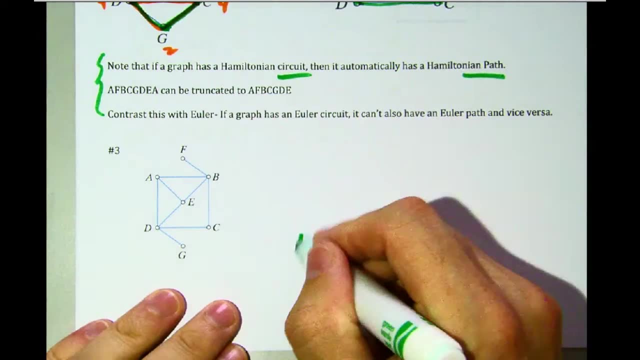 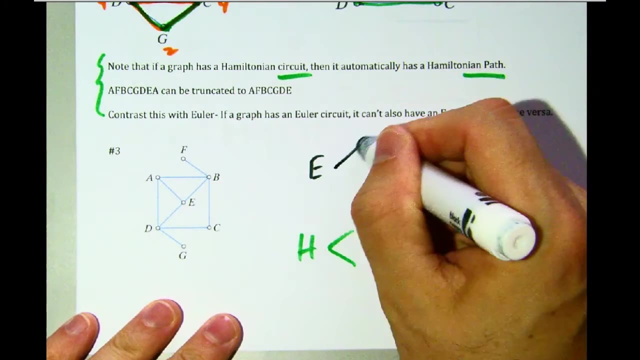 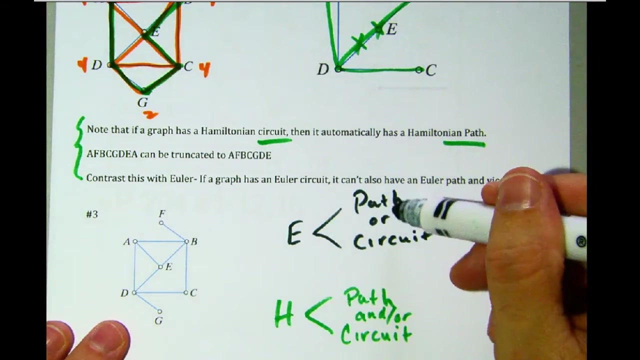 is also a path once you try number three and see if you can find Euler and Hamiltonian path and circuit and bring that to class and we'll see what you said about both of those. okay, so tell me, is it gonna be a path or circuit for Euler and then path and or? 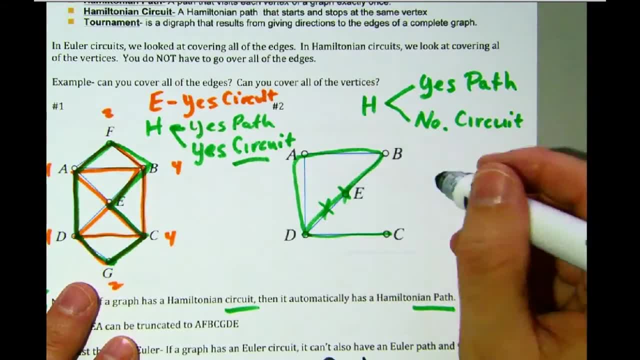 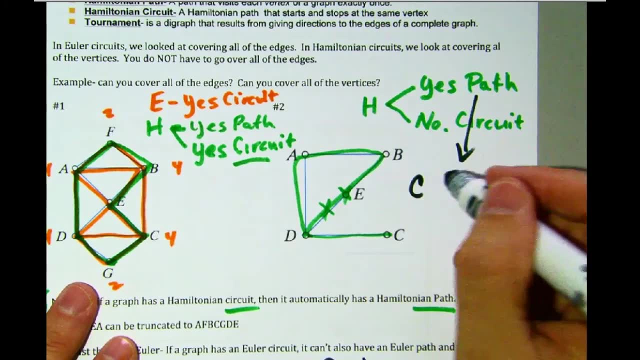 circuit for a Hamiltonian. let me go back to this one. if I wanted to write out this path, what I would do is- I said that I started at C. I can just write it out: C, D, A, B, E. this would be my Hamiltonian path. okay, this is how we write these out. 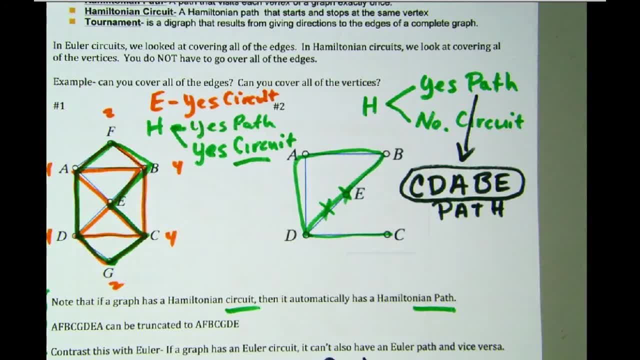 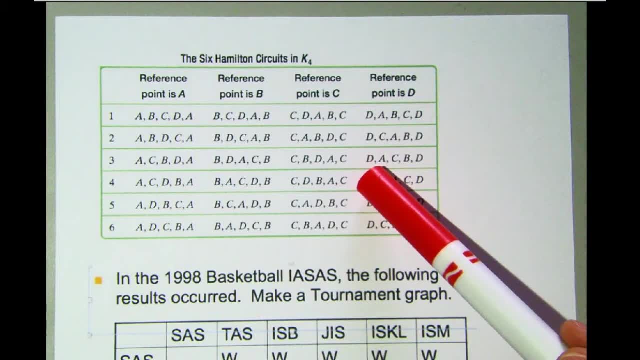 tell me where you start, tell me where you finish. no problem there. okay, let's go to the next page. this next chart tells me how many different Hamiltonian circuits I can have in a k4. we'll talk about this in class, so ask me about the k4 and the not different number of Hamiltonian. 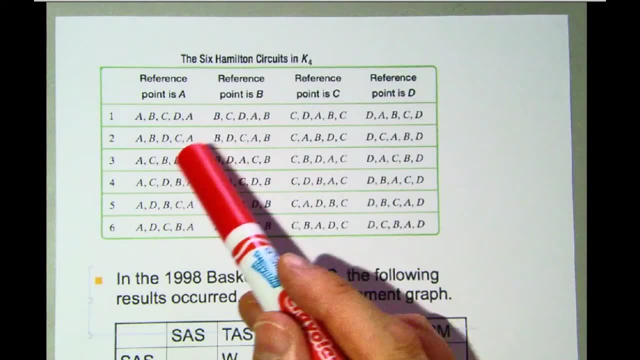 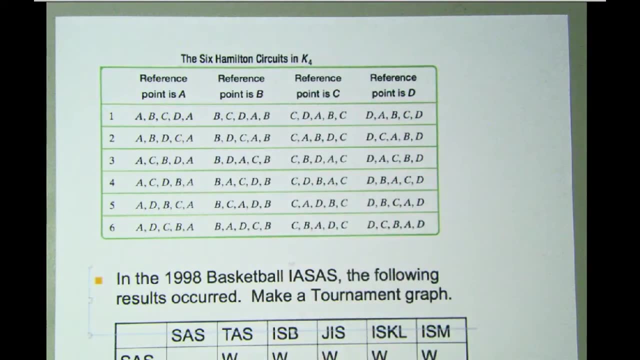 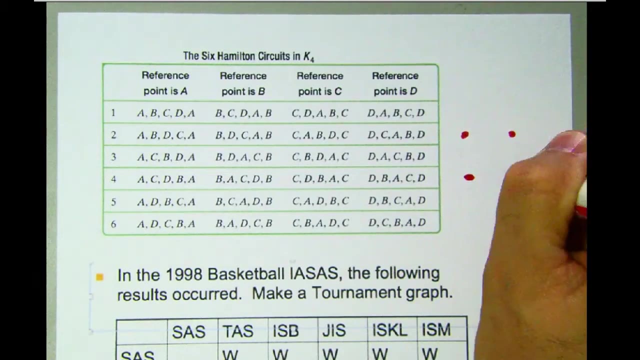 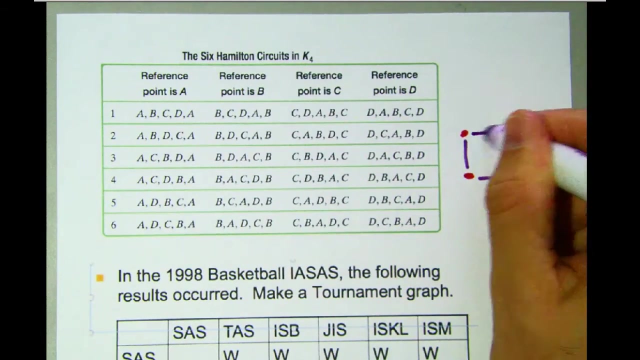 circuits you can have, so in other words, if one person does this, they might get this one here, another person does it, they might get this one here. however, both of you have a Hamiltonian circuit that you did make up for the k4. remember that the k4 is the complete graph for four vertices. that's the k4. okay, now the 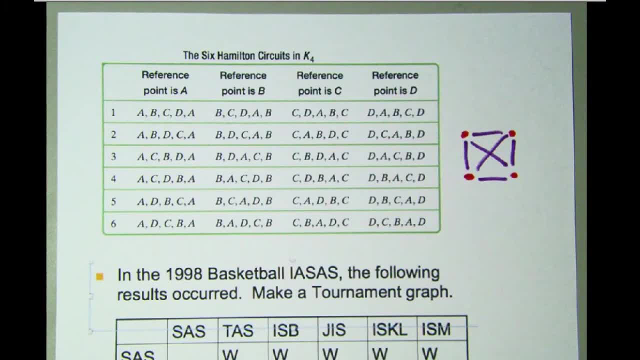 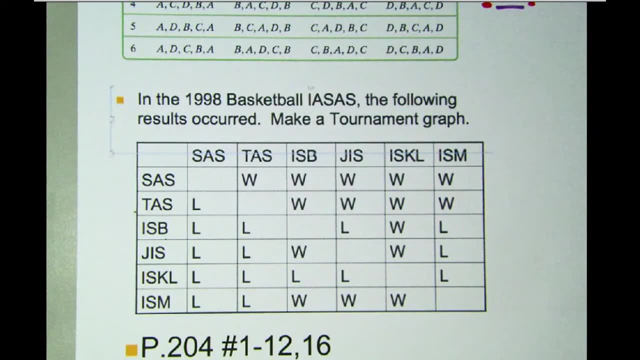 last thing we want to do in this section is look at a tournament and build what we call a diagraph. so what we have is in the 1998 basketball. I made this up so this isn't true. sorry if anybody's checking me. basketball, I asked: is the? 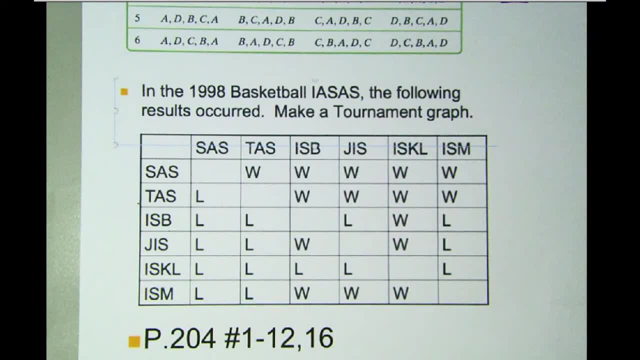 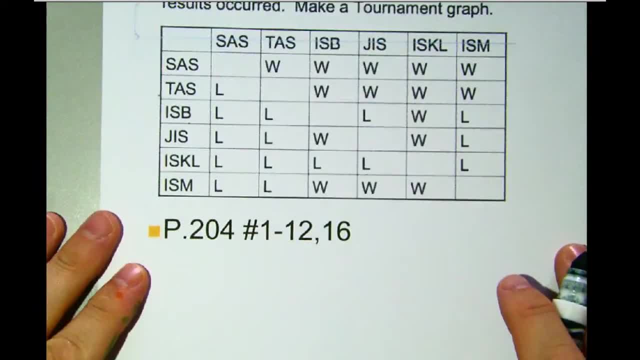 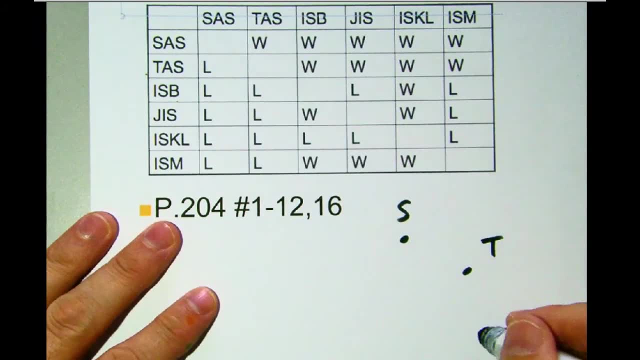 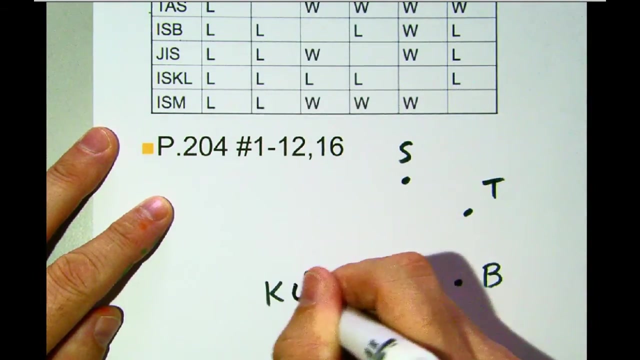 it. so you're going to start off with each one of these schools. so I have SAS, I have Taipei, I have is B, I have GIS and I have that's off the board. there we go. and then I also have a ISKL, and then I have ISM. so that's how I 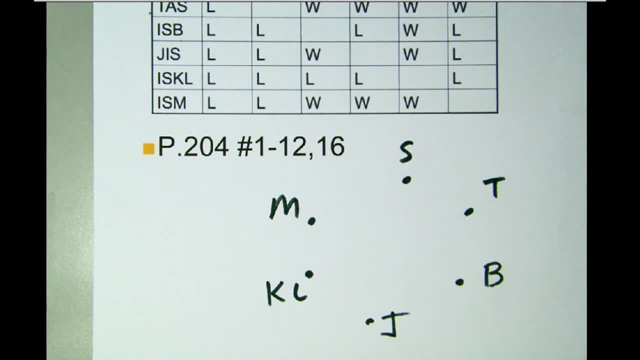 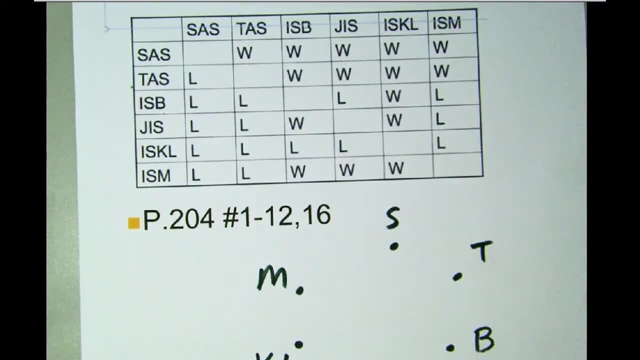 graph that. now what's going to happen is that in a tournament graph, you are going to make a diagraph, so you're going to do arrows wherever you have a winner. so this is written with respect to these teams, right here. so when I write a W, 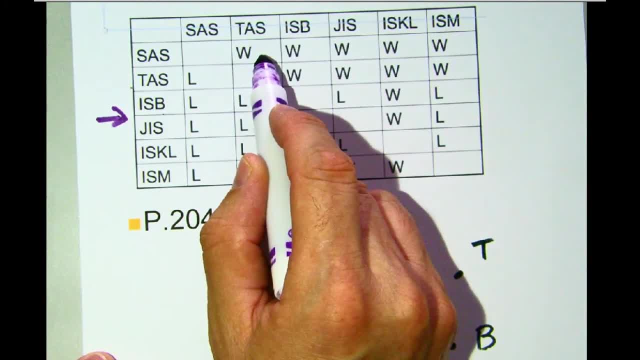 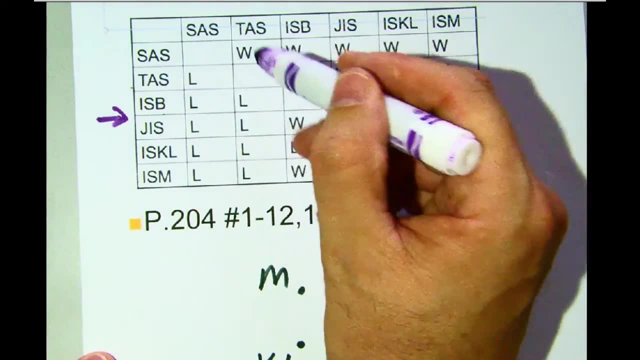 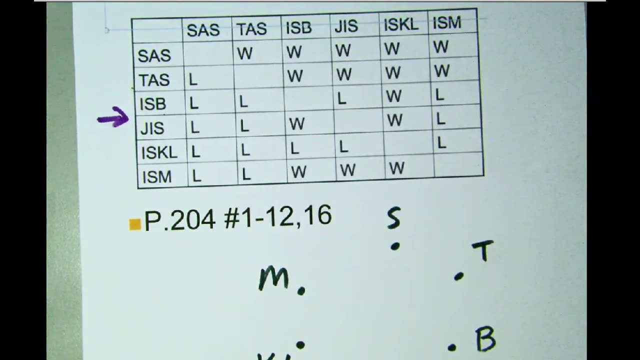 right here. that means that SAS beat Taipei, and so on. Taipei has an L here, so then that means they lost to SAS, and so this has kind of a reverse symmetry to it. if you go opposite side, a W turns into an L over on the other side. I did that wrong. this one, this one, matches up with this. 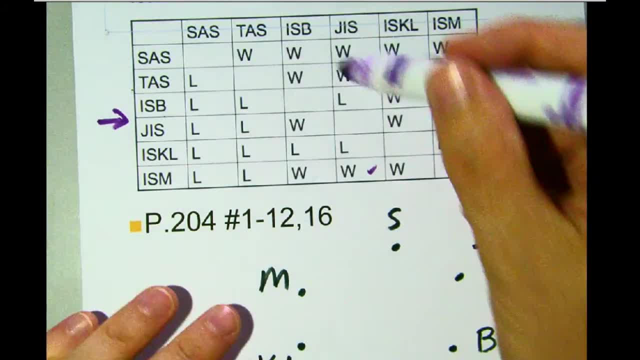 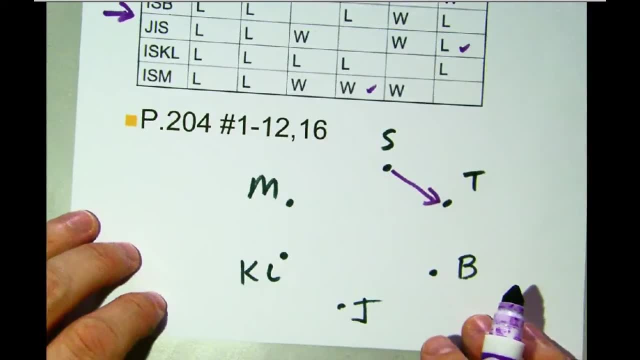 one W matches up with an L. so what happens now is that SAS beat all of their opponents. so when you beat somebody, you're gonna draw an arrow to them. so that's what I'm going to: draw an arrow to them. so that's what I'm going to. 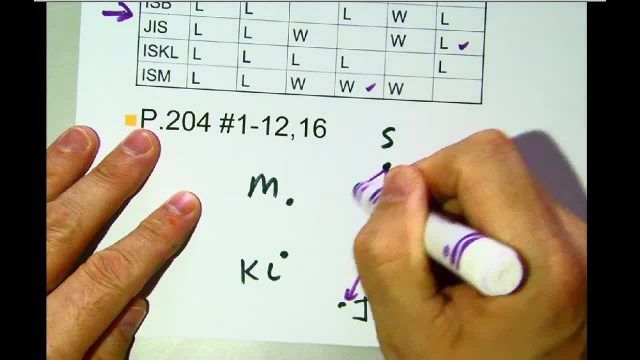 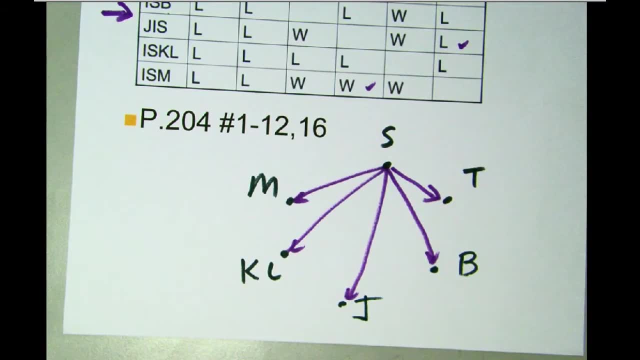 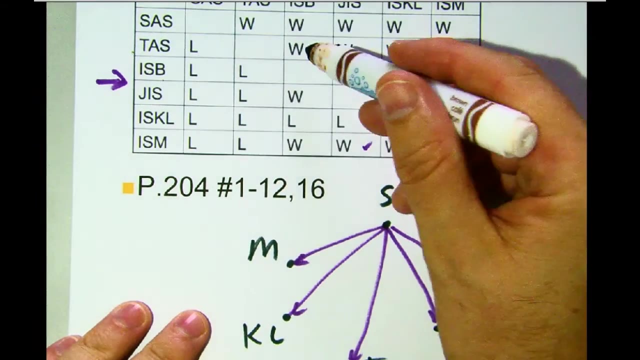 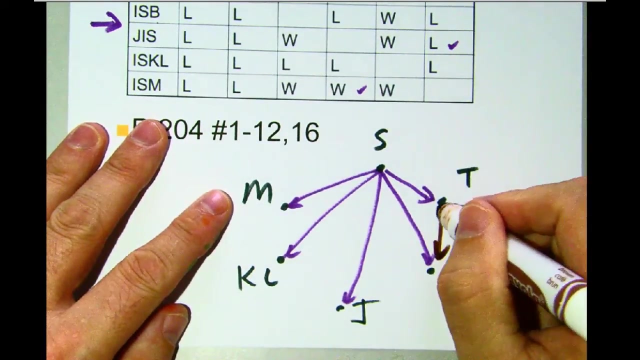 do for all of these? SAS beat each one of their opponents. now, if I move on and I look at Taipei next, I'm just going in kind of an order: who picked who had the most wins? then Taipei beat everybody except for SAS. so when I do this, 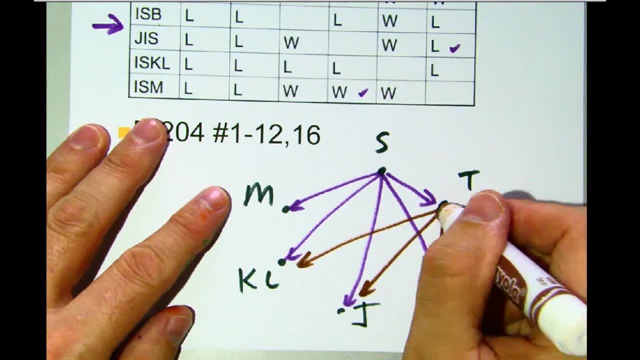 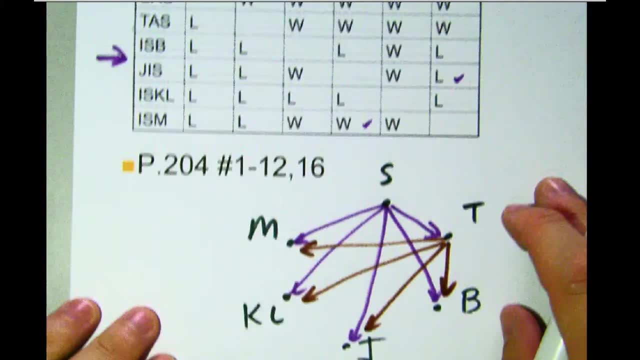 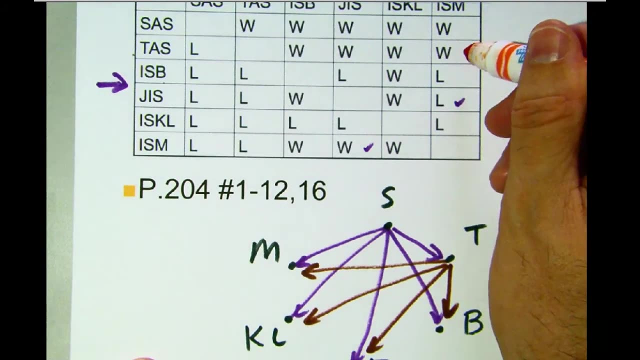 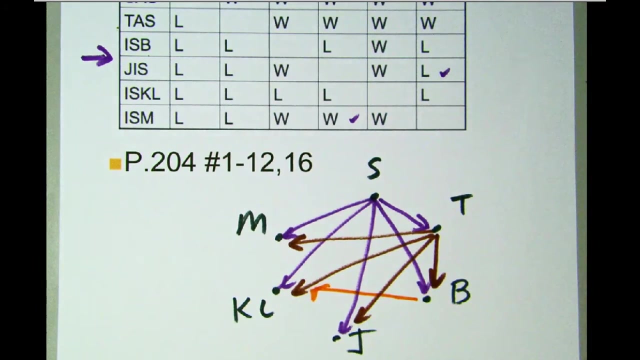 I don't go back to SAS because they only played one game, so it's going to be a complete graph with no multiple edges. and then, if I go to ISB, double-check me if I'm doing this right. ISB ended up just beating KL, so I get that there, and then also I have JIS. 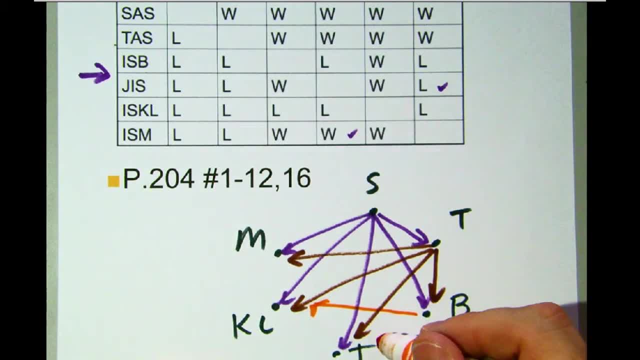 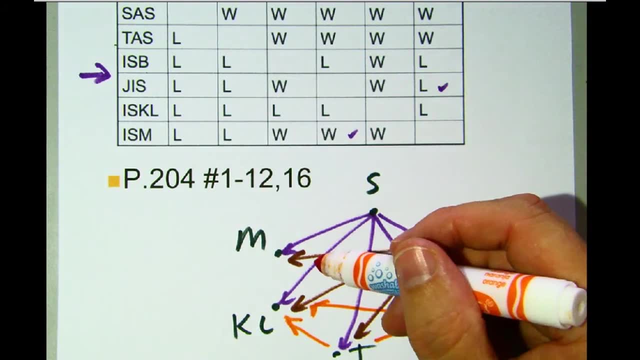 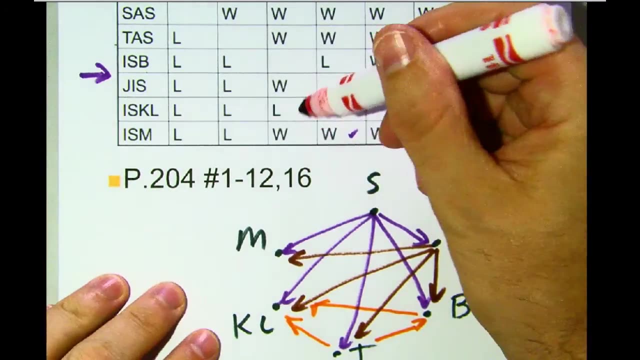 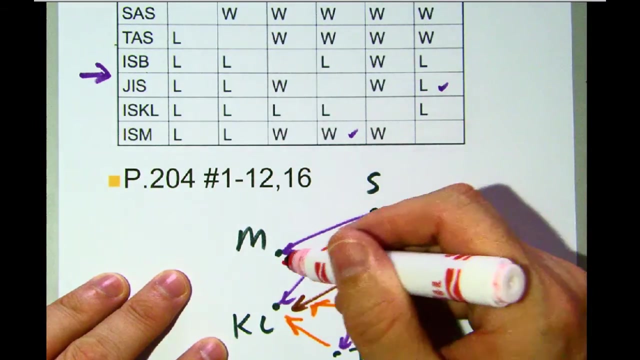 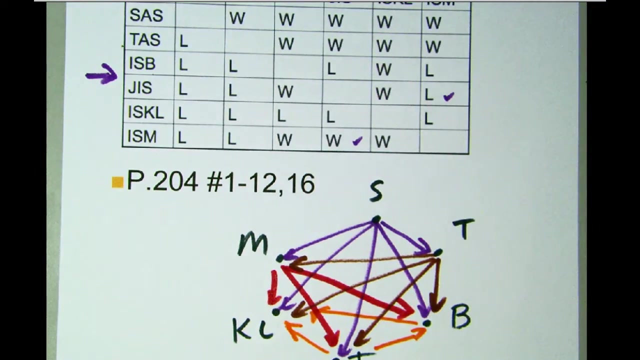 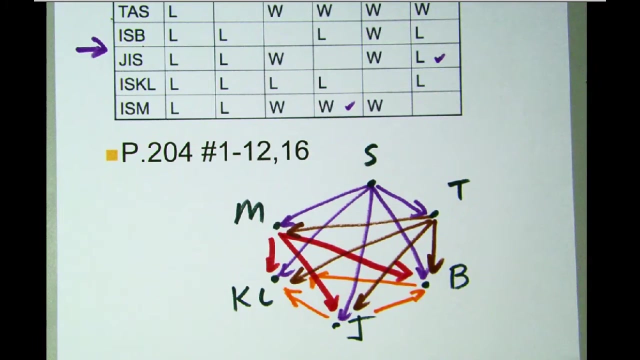 JIS beat ISB and JIS also beat. I ask: helps. and ISSM then beat. good baby. now ISM beat ISB, I and ISM beat. yes, ISM beat ISKL. 구요 happens now is that, if I did a Hamiltonian path here, which vertex would I have to start at? 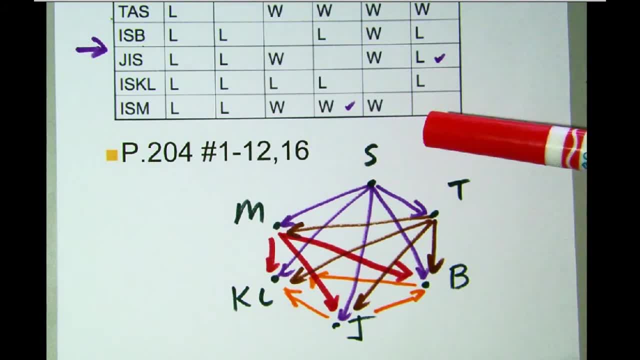 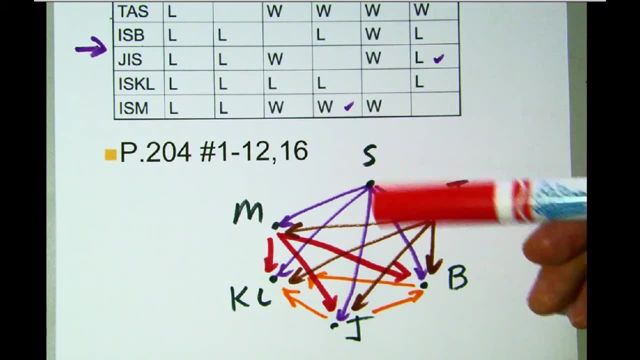 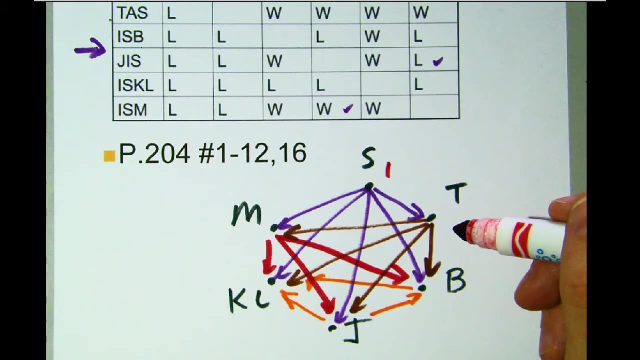 I hope that you can figure out that you'd have to start at SAS. I can never get back to SAS, so I'd have to start here. so this is my starting point. now I can figure out different paths. in fact, I want you to see if you can figure out a path. so pause this, see if you can start at SAS and get all. 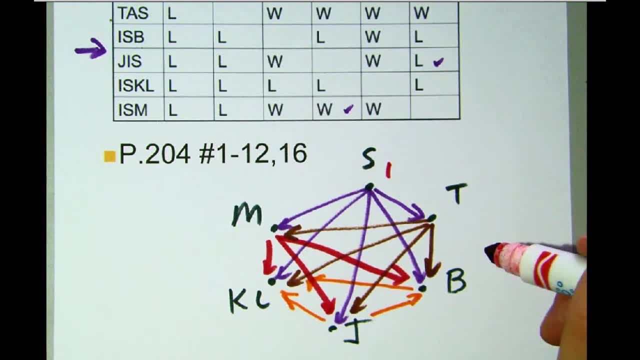 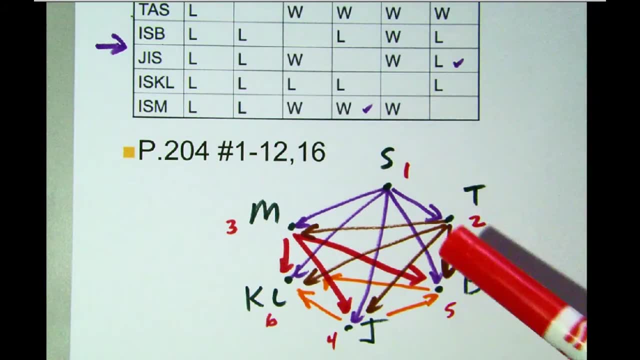 the way around following the order of the arrows. pause this now. if you notice, I wrote down the order here. hopefully you tried this and went through this SAS to Taipei, to Manila, then I have to go over to nope, down here to Jakarta and then over to Bangkok and finish.